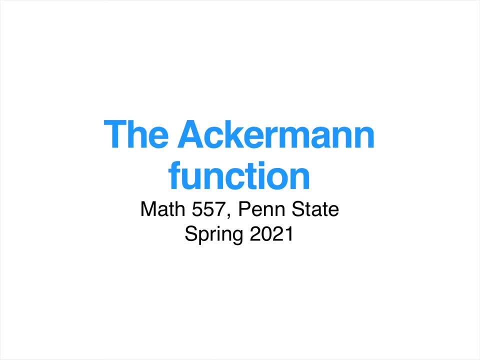 In this brief video we give a short introduction to the Ackermann function, which is important from a foundational point of view and also because it kind of introduces us to the growth behavior of functions on natural numbers. So the Ackermann function arose as an example of the search for a computable function. 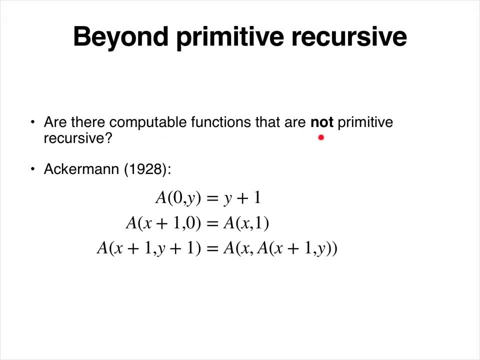 so a function which is intuitively computable, that is not primitive recursive, And Ackermann was a student of Hilbert and in the late 20s gave a following example: So it's a binary function. so a of 0, y is y plus 1, a of x. 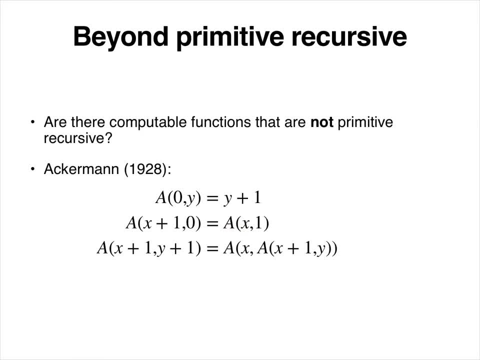 plus 1, 0 is just a of x comma 1, and now here we have a double recursion, So a of x plus 1, y plus 1 is a of x, of a of x plus 1 comma y. It may not be immediately clear. 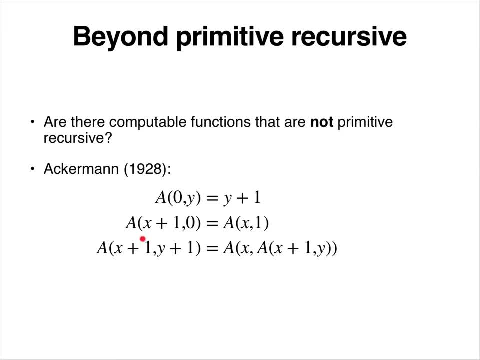 that this recursion here actually gives us some computable function, in particular when we try to unravel this right and compute this value by using this recursion property here that we actually terminate after finitely many steps. But you can see that if you apply a 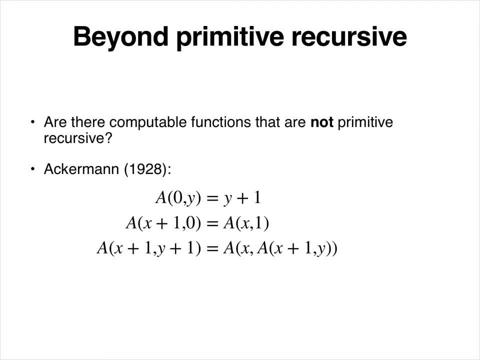 recursion step. you either x, so x plus 1 goes down to x, or x plus 1 here stays the same, but then y goes down. So in particular you always go down in the lexicographic ordering right, and that's a well ordering. on the pairs. on the pairs. 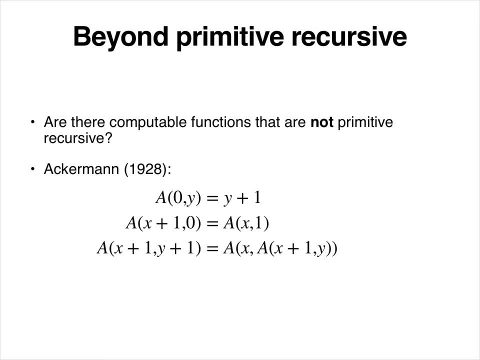 On the set of finite pairs, and hence, after finitely many steps, you must have reached the part where you have a well-defined expression here, or number, So showing that this is actually formally computable in the sense of Turing computation or other computational frameworks. 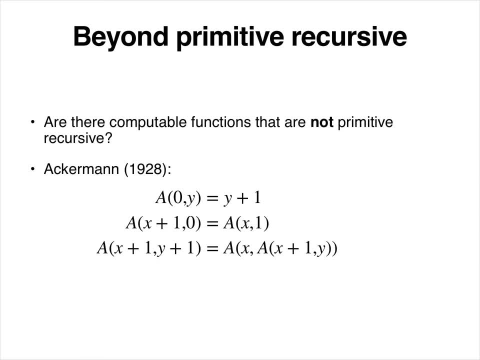 is quite a little bit harder And we will discuss this later. Subtitles by the Amaraorg community Later as an implication, for example, of the recursion theorem. For now we want to focus on an aspect of the Ackermann function. So, assuming that this is, 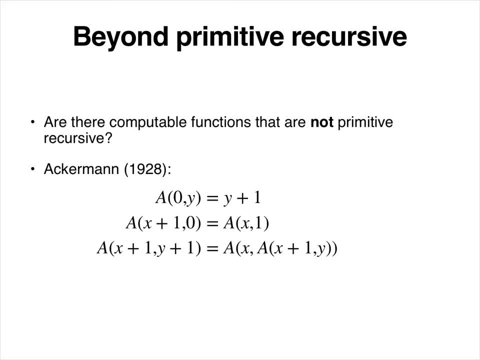 an informally computable function right that it is actually not primitive recursive, You see here. so this definition uses a double recursion. The definition of primitive recursion only had a simple recursion right in the second component. So why is it not possible to express this maybe as a 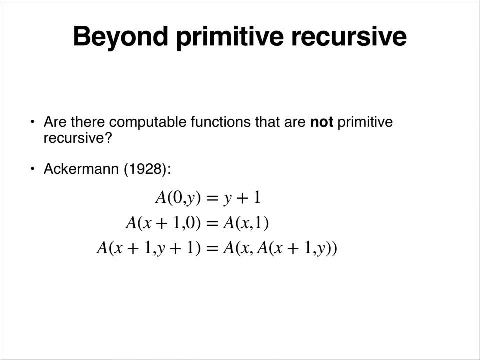 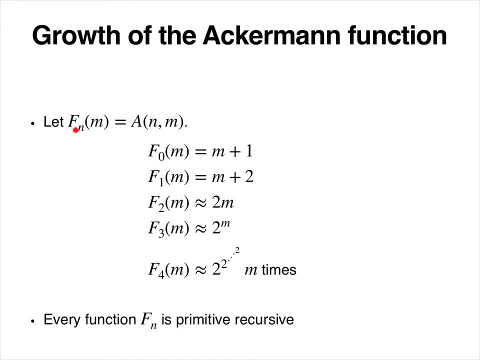 more elaborate, simple recursion. The reason is the growth behavior of this function that we'll describe on the next slide. So let's assume let's fix f sub n, So fix the first component of the array function, because the style function has only fr. 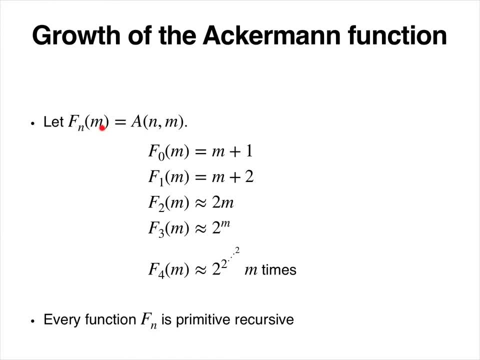 Ackermann function right and look at it as a unary function in the second component And then you should try that for the first few values and you will see that the first function, so the first component function, is m plus 1,. the second component function is m plus 2,. 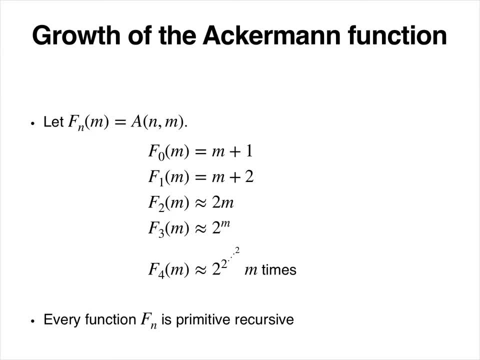 then f sub 2 is approximately 2m- it's off by a little bit. and then the third f sub 3, is 2 to the m. f sub 4 then is a tower of the exponent: 2 to the 2 to the 2, and so on m times. 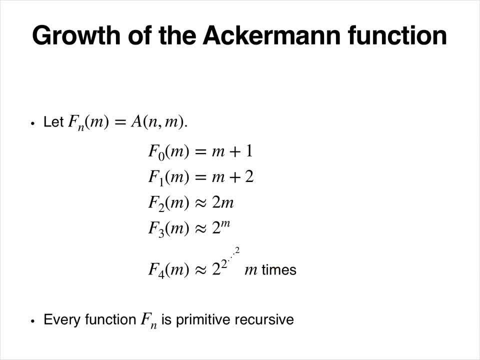 So what you see is that the Ackermann function essentially iterates the basic operation. so it iterates plus 2 times, then it iterates times to exponential, then it iterates passing from f3 to f4. It iterates exponentiation, and so on. 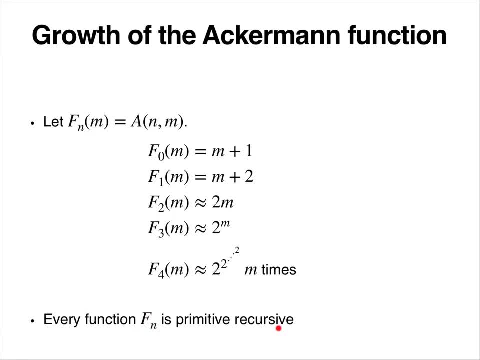 You can also show that every function fn is actually primitive recursive. so if we fix n, we get a primitive recursive unary function. But you can also observe that now in the first component. if we fix the second component and look at the first component, we get an extremely fast or growing function.